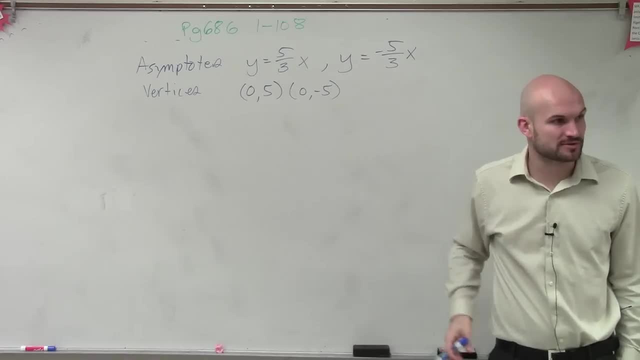 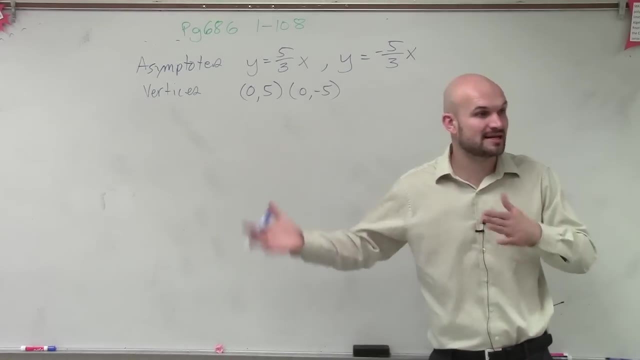 to keep on saying this, I need to figure out which equation I'm going to use. There's one equation where it's x minus h minus y minus k, and the other equation is y minus k minus x minus h. So I need to figure out which one I'm going to use, for a horizontal or a. 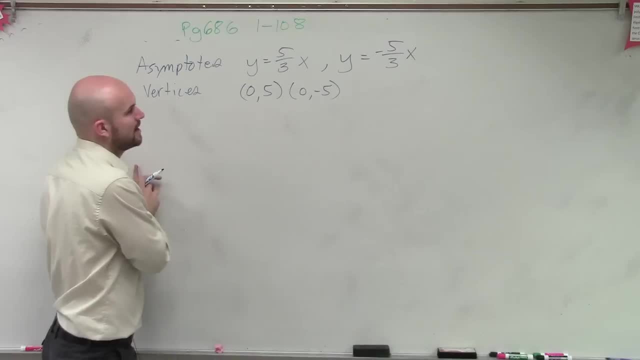 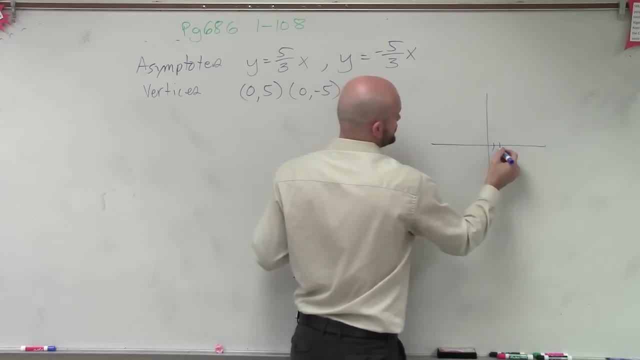 vertical. The only information I'm given right now is 0, 5, and 0, negative 5 are the vertices, So let's plot them: 0, 5 is 1, 2,, I'm sorry. 0, 5 is 1,, 2,, 3, 4, 5, and 1, 2, 3, 4, 5.. 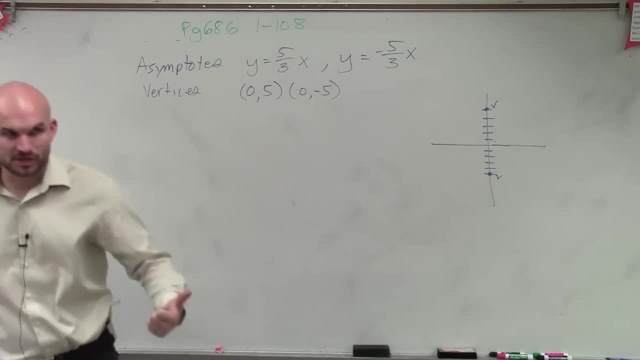 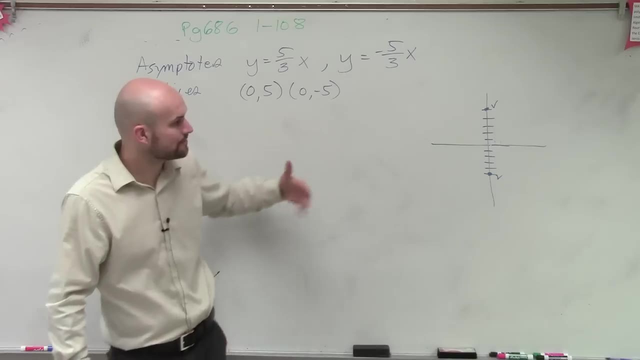 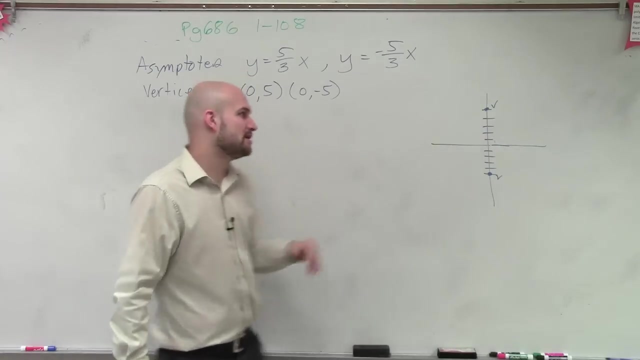 Now, those are your two vertices. We know our vertices, our center and our foci all lie on what we call the transverse axis, right? So is our transverse axis then vertical or horizontal Vertical? So the formula for a vertical transverse axis is going to be- remember it's always a squared- 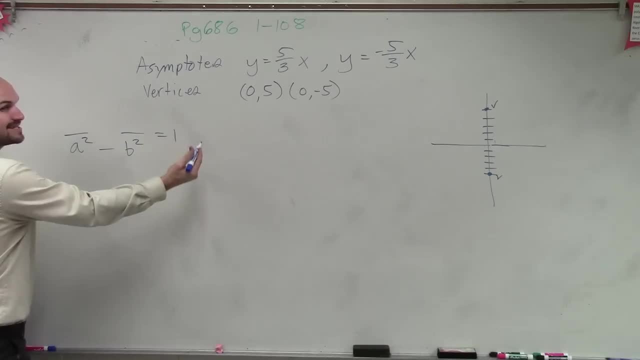 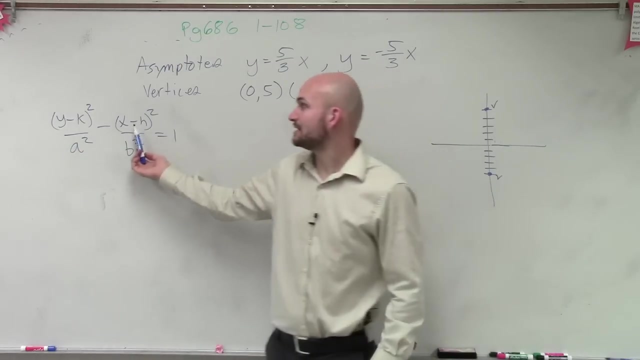 minus b squared as your denominators, right. But since now it's vertical, I'm going to have y minus k squared. So I'm going to now use the other form of our formula. When we have a vertical transverse axis, our y squared is over our a. If it was a horizontal transverse axis, the x minus. 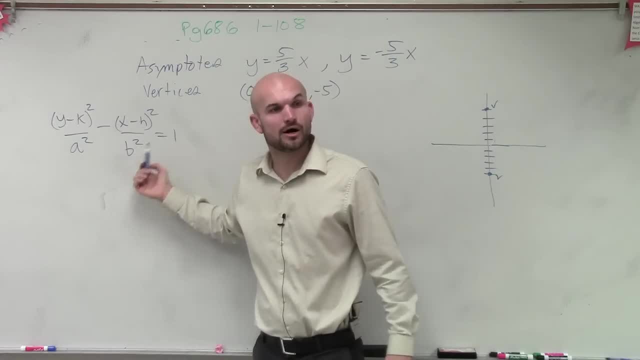 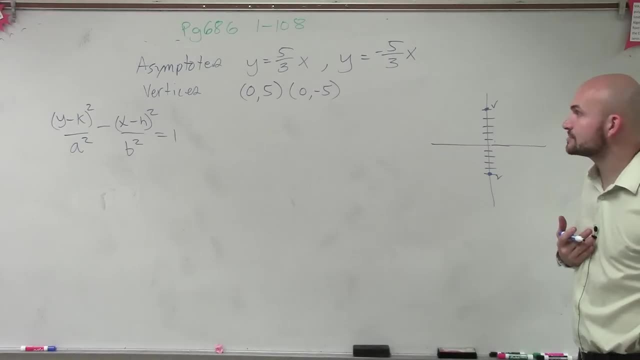 h squared would be over the a, but it's always a squared minus b squared, always for a hyperbola. Okay, so now we need to determine what our a, b and c are right. So first of all, 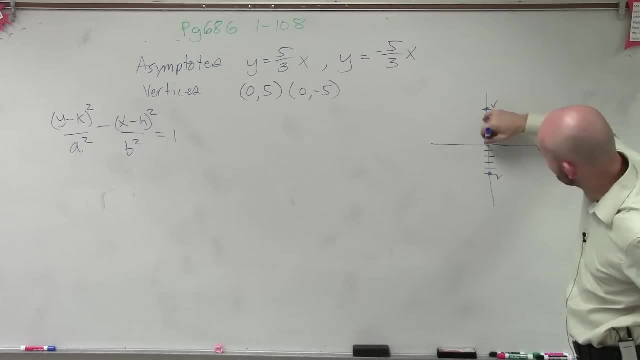 our vertices. remember the distance from your vertice to your center is a Well. first of all, let's figure out what our center is. We know that the center is equidistant away from our two vertices. right, The center is right in the middle, So you guys could use the midpoint. 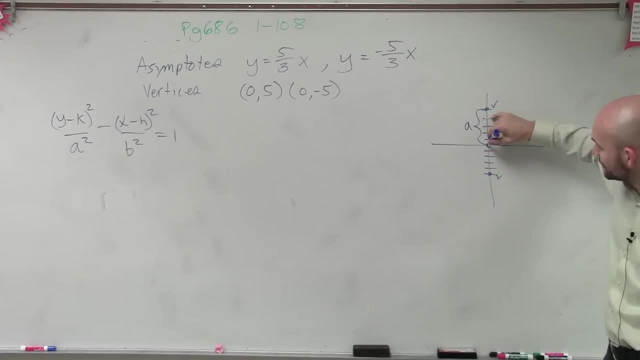 formula if you wanted to, or you can just look at it and say: alright, the center is zero comma zero, right, And since our center is zero comma zero, we know our distance. a has to equal b, a, b.